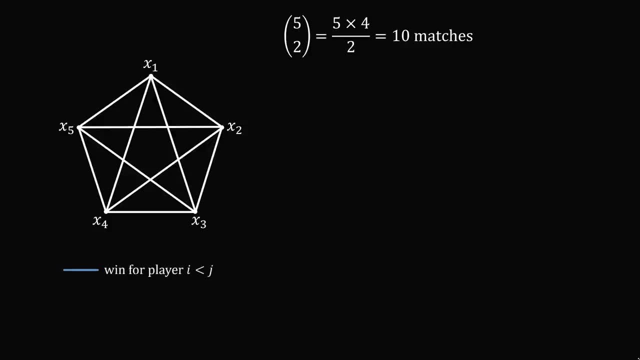 Now let's color these edges. We can color an edge blue if it's a win for player i less than j, and we'll color it red for a loss. So each of the different edges have two different colorings. So the total number of possibilities is equivalent to the total number of colorings. Now we have 10. 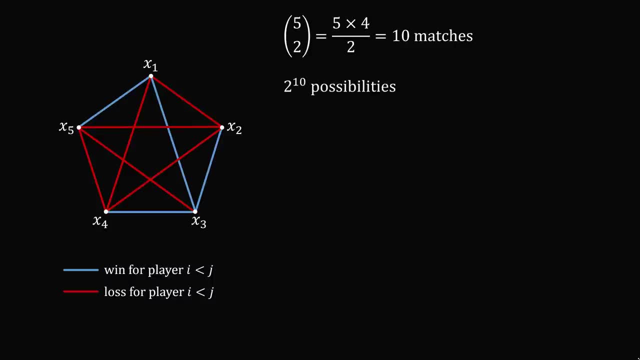 edges with two different possibilities for each one. So that will be 2 to the 10 different colorings or 2 to the 10 different possibilities for the outcomes of these matches. Now let ei be the event. xi wins all four of her games. So let's calculate the number of elements in e1.. Now, from: 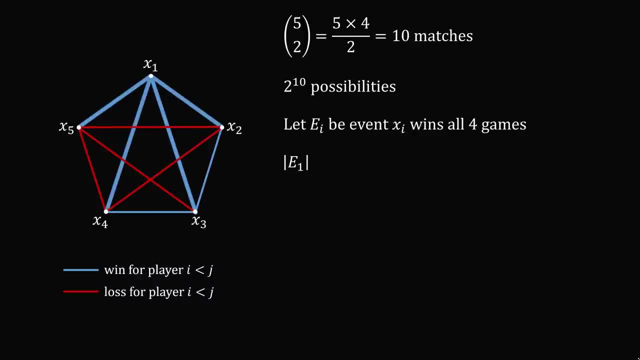 node 1. we need all four of these edges to be colored blue. There's only one way to do this. Now there are six remaining edges, and each of these edges can be colored either blue or red. So that will be 2 to the 6 different. 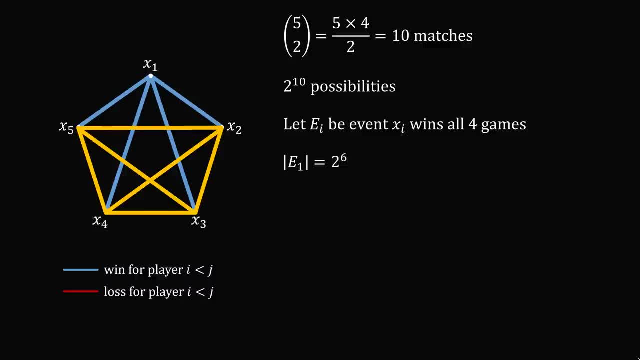 ways we can color these edges. So the order of e1 is equal to 2 to the power of 6.. Now, by the same logic, that's true for any of the other players. So we can calculate the order of e2,, e3,, e4, or e5. 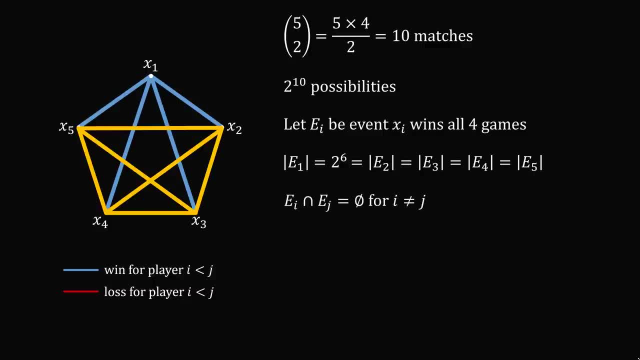 Now here's a key part of the problem: Ei and ej have an empty intersection. So if player 1 wins all of her games, since player 1 has played all of the other players, that would deal a loss to all of the other players. So it's not possible that one of the 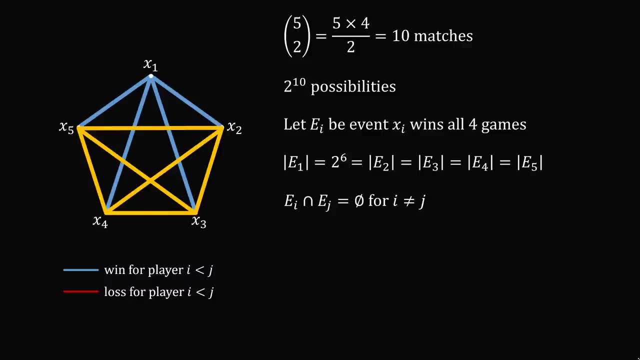 players wins all their matches and some other player wins all of their matches. It must be that these are mutually exclusive events, So now we can count this. So we want the total number of e1,, e2,, e3,, e4, and e5 divided by the total number of possibilities. 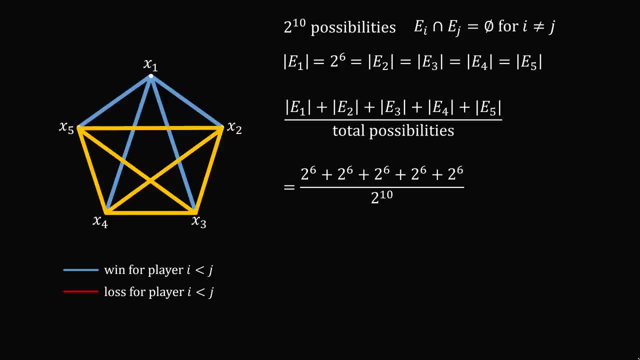 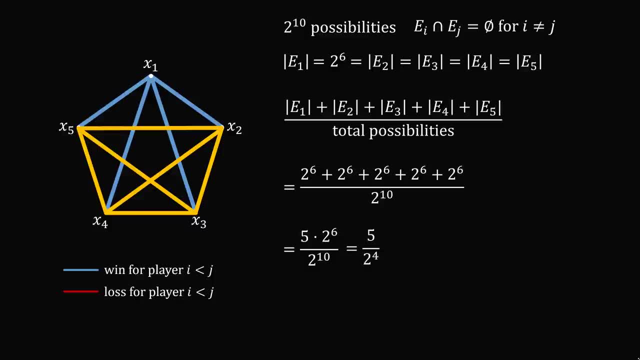 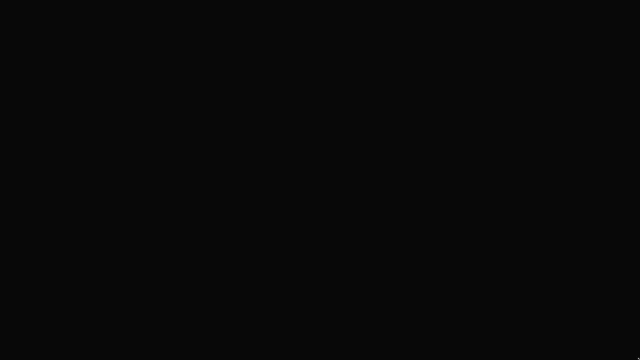 which equals 5 divided by 2 to the power of 4.. And that gives us the answer of 5 over 16.. Wow, So now let's do a shortcut and solve it in a quicker way. We'll use the same notation as before. 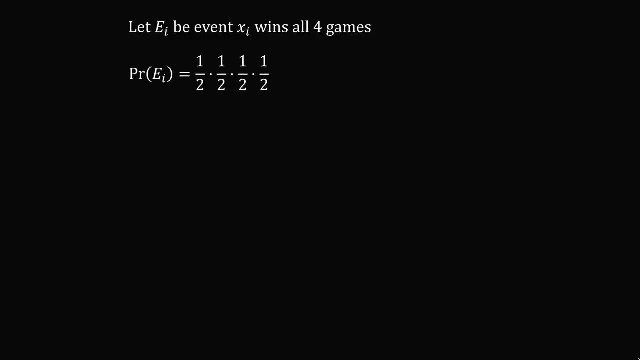 Now what's the probability that some player wins? The probability that a player wins all four games, it'll be one half times one half times one half times one half, because each of the four games has a probability of one half of winning the game. 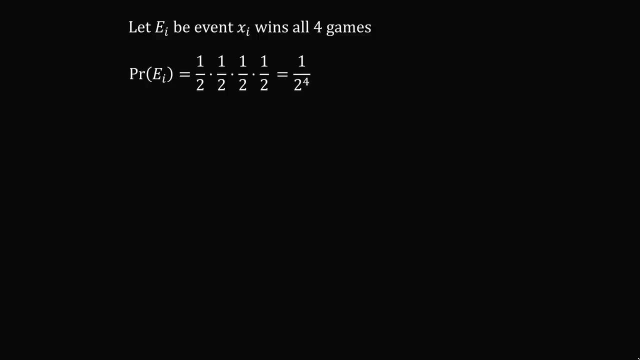 So this is equal to 1 divided by 2 to the power 4.. Now, as we argued before, eI and eJ have an empty intersection, So we want the probability of the union of e1 to e5.. Since the events are mutually exclusive, this will be the sum of the probabilities. 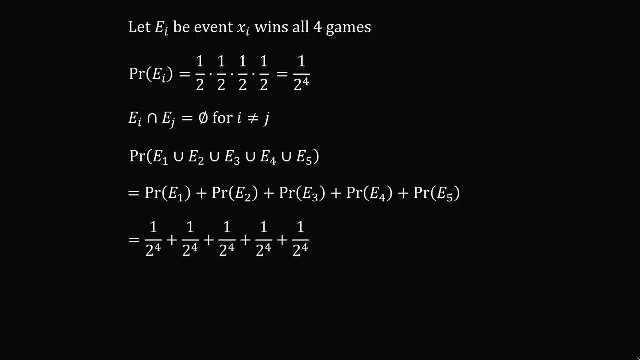 of each of the events. Each of the events has probability 1 over 2 to the power of 4, and this is true for five events. So this will be equal to 5 divided by 2 to the power of 4,. 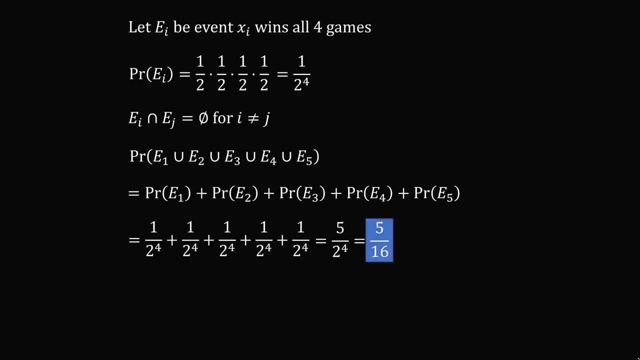 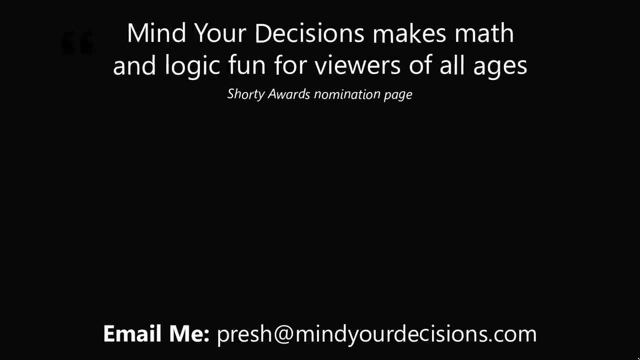 which is equal to 5 over 16.. And that's the answer. Thanks for making us one of the best communities on YouTube. See you next episode of Mind, Your Decisions, where we solve the world's problems one video at a time. We'll see you then. 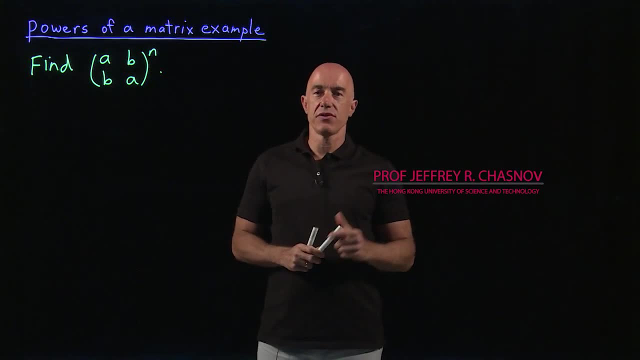 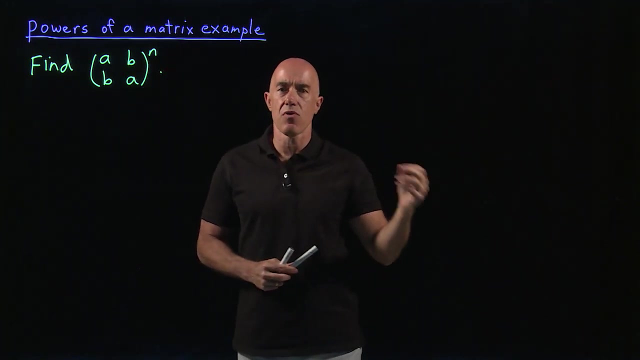 So in the last video I showed you how we can use matrix diagonalization to find a matrix to a very large power. I think we should be concrete now. so let's start with the matrix we already diagonalized and let's compute that matrix ABBA then raised to some arbitrary 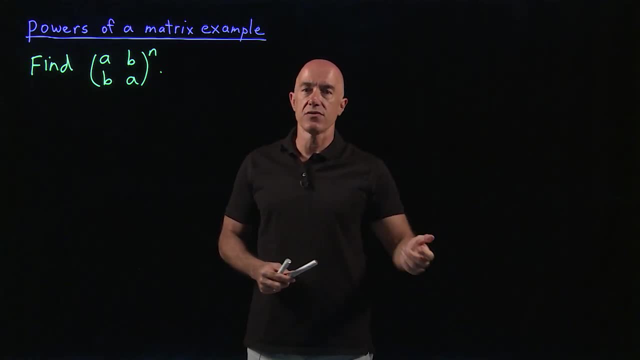 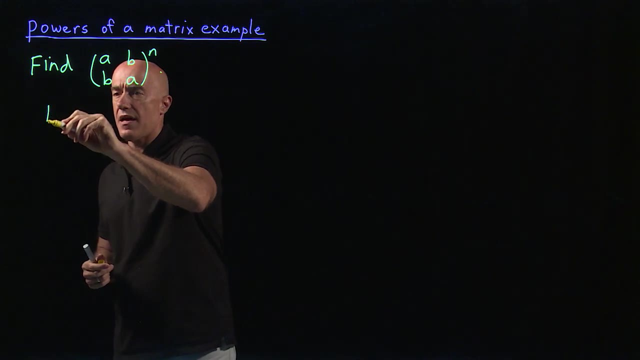 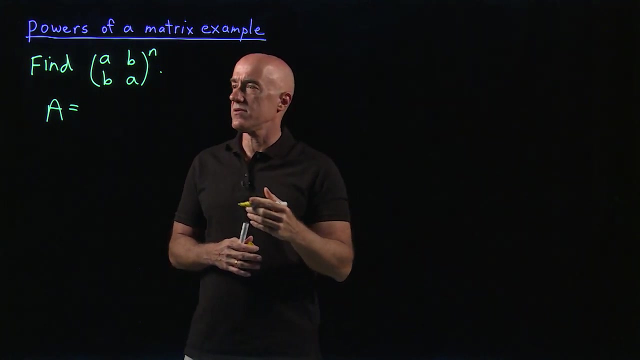 large power, N. So N can be anything. we want 1,000,, 2,000.. So we have to. so we're using the idea that this, any matrix A, well, a matrix that has N linearly independent eigenvectors.